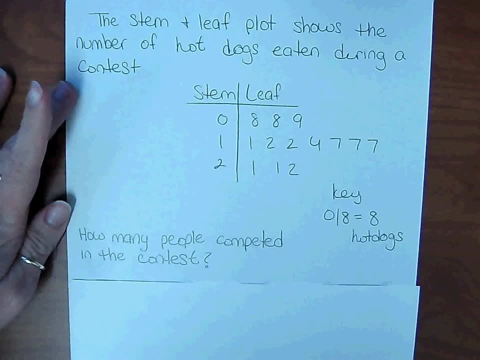 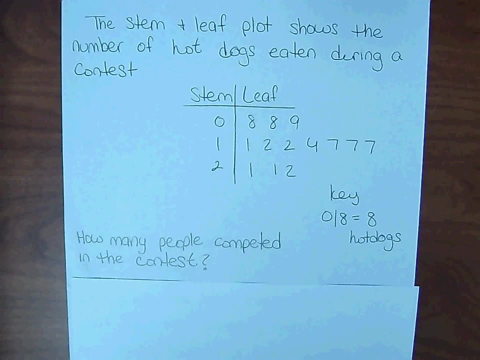 How many people competed in the contest? Well, if the stem and leaf plot shows the number of hot dogs eaten during a contest, 8 hot dogs was eaten by one person, and then another person ate 8,, and another person ate 9, and so on. 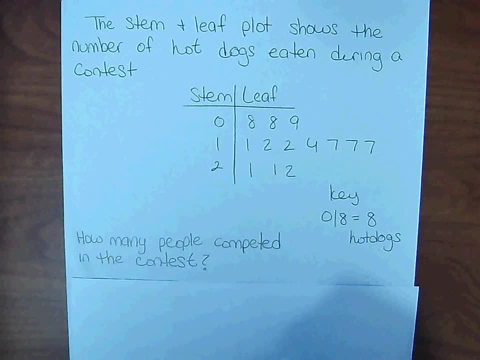 So if we count each piece of data, we'll know how many people competed in the contest. So 1, 2, 3, 4,, 5, 6,, 7,, 8,, 9, 10.. 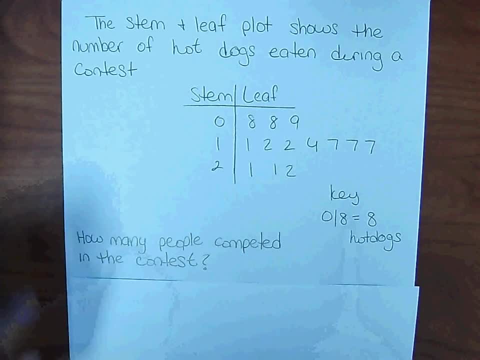 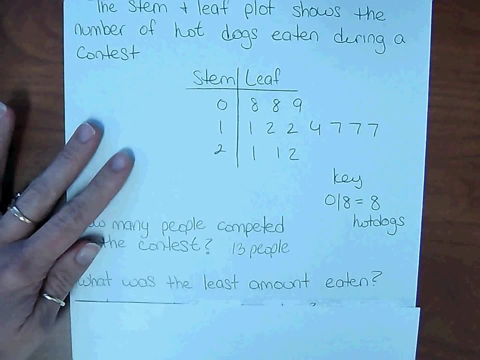 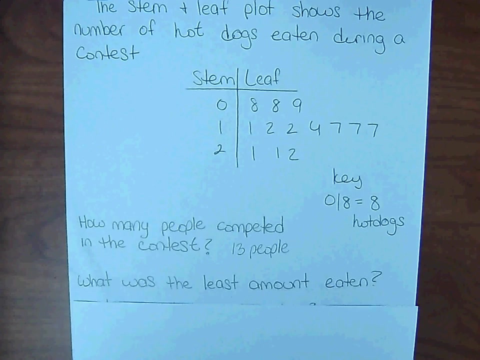 11,, 12,, 13.. So 13 people competed in the contest. What was the least amount of hot dogs eaten? Well, the least amount would be the smallest stem and the smallest leaf. So 8 hot dogs is the least amount eaten. 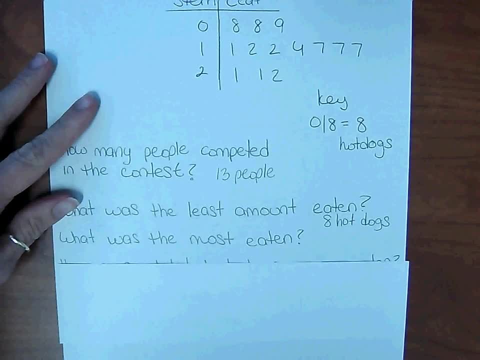 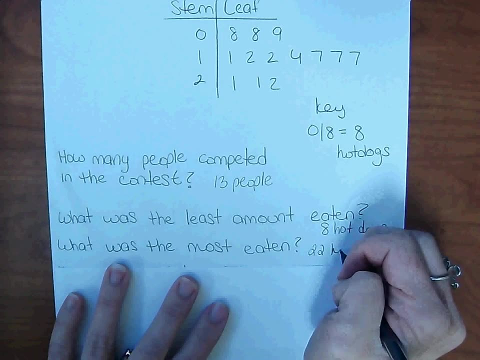 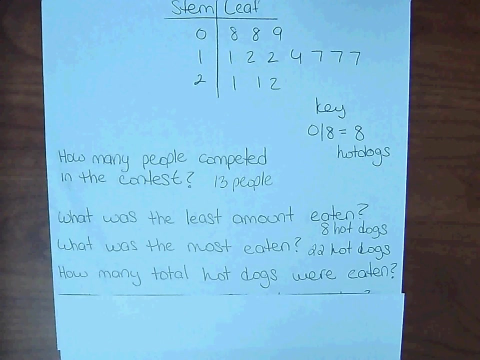 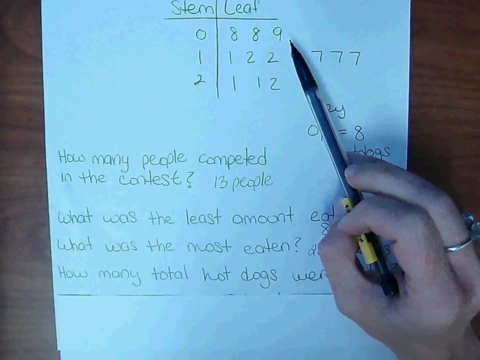 What was the most amount that was eaten? Well, that would be the biggest stem and the biggest leaf, So 22.. How many total hot dogs were eaten? Well, we know 13 people ate them. One person ate 8,, one person ate 8,, another person ate 9, and so forth. 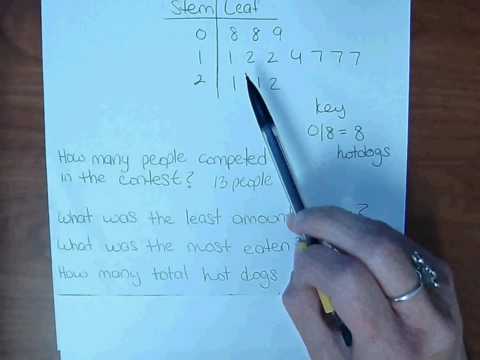 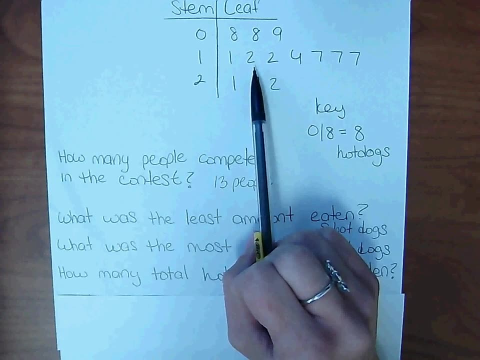 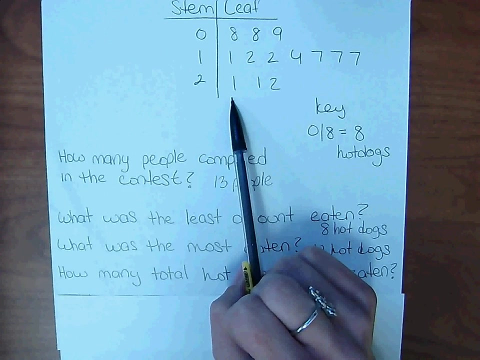 So to find out how many hot dogs were eaten, we need to add up all these numbers, So 8, 8, 8,, 11,, 12,, 12,, 4.. 12,, 14,, 17,, 17,, 17,, 21,, 21, and 22.. 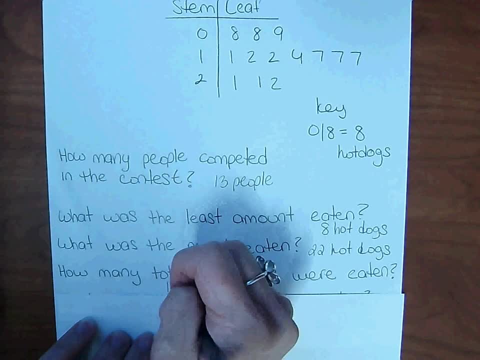 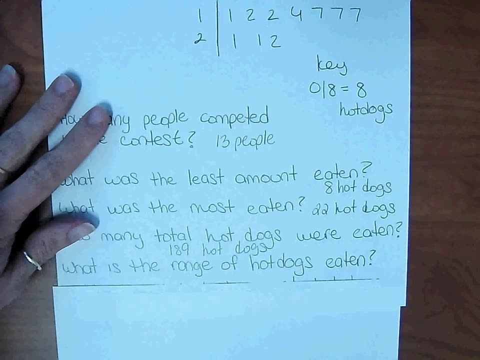 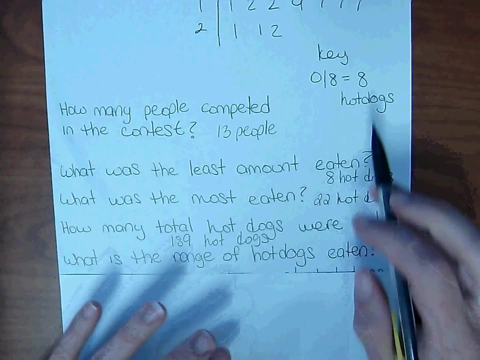 So in this competition, 189 total hot dogs were eaten. What is the range? Well, range is the highest minus the lowest, So the highest is 22.. And the lowest amount eaten is 8.. So the range is 14..